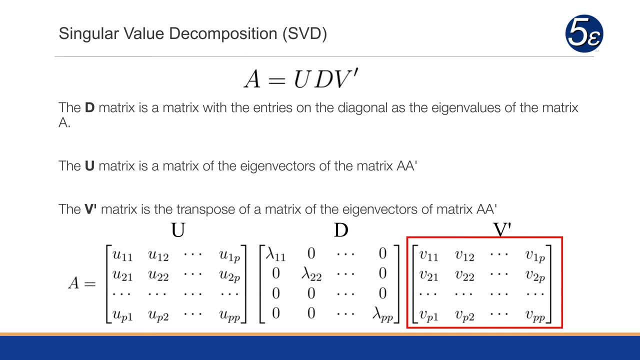 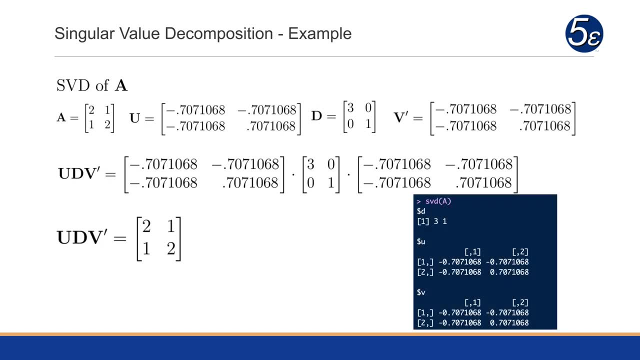 eigenvector matrix of A times A transpose. So this gives us our u, d and v matrix. So here's an example of our Singular Value Decomposition. We have our matrix A as 2, 1,, 1,, 2, and we compute.